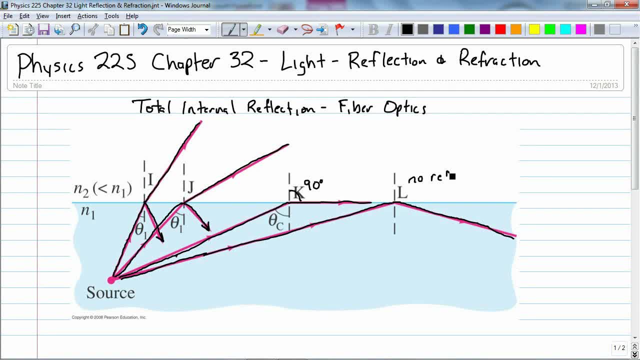 And this is total internal reflection. Now we can use Snell's Law to figure this out. We have n1 sine theta 1 is equal to n2 sine. but if I want to know the critical angle, that sine is going to be 90 degrees And sine of 90 degrees is 1, so I'm going to have the 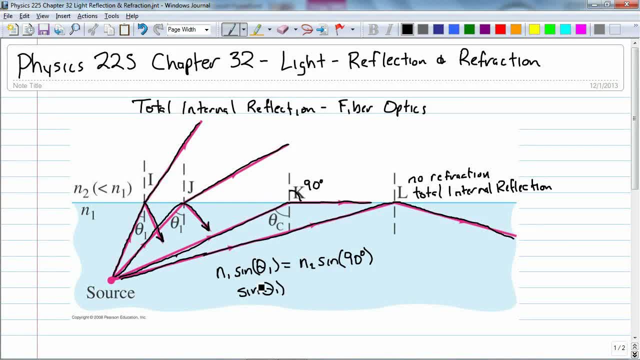 sine of theta 1.. And that sine of theta 1 is equal to n2 over n1. And this n2 over n1, because n1 is greater than n2, is going to be less than 1, which I need for the arc sine. 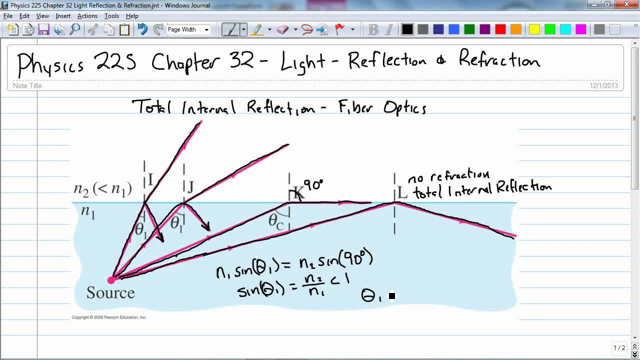 So theta 1 is equal to the arc sine of n2 divided by n1.. theta 1 is equal to n2 over n2.. And theta 1 is equal to n2 over n2.. And theta 1 is equal to n2 over n1.. 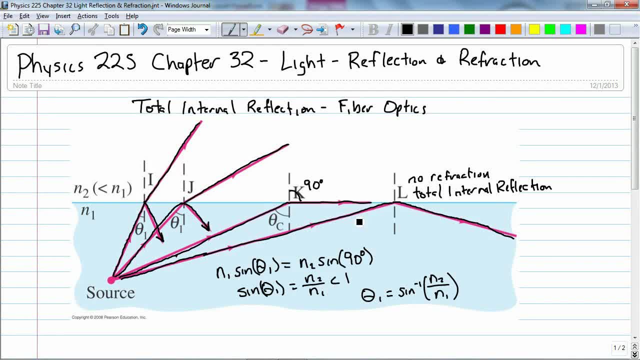 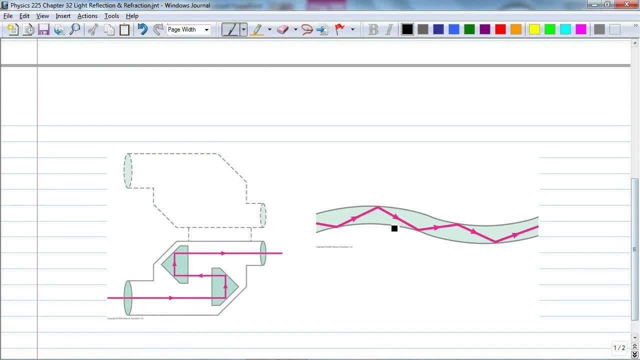 When theta1 is greater than that, I'm going to have total internal reflection. Now we can use this idea for different applications. One would be binoculars. You have these total internal reflections based on how these crystals are shaped and their refractive index. 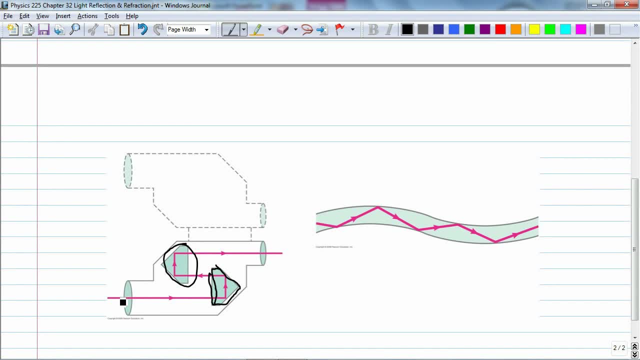 To guide light from the view lenses to the eyepieces. In the case of fiber optics, you get total internal reflection based on these refractive indexes And because of the total internal reflection, very little light gets out of fiber optics, Which makes it a fairly good medium to transmit information from point A to point B.